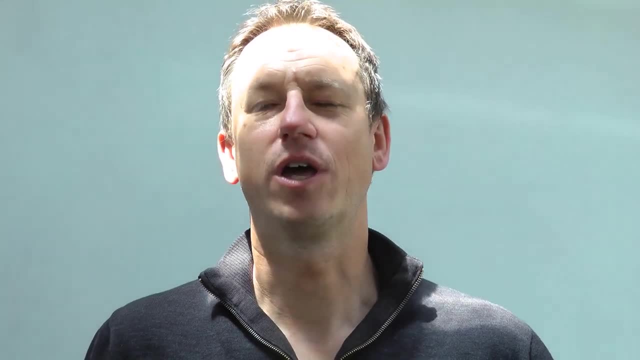 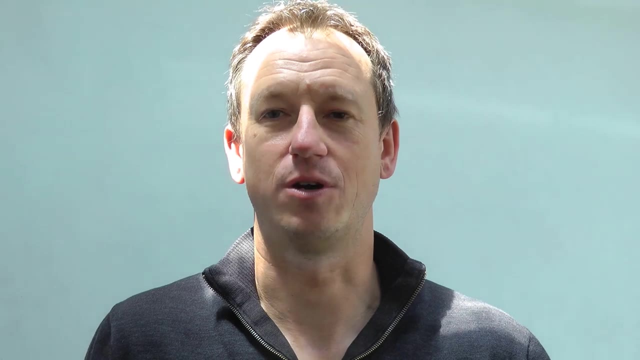 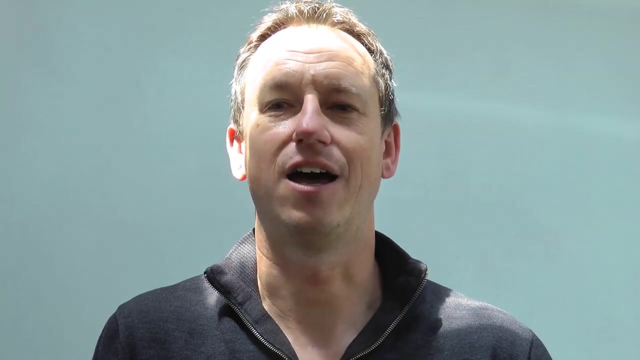 Hello friends, and welcome to A Shot of Code. Today we're going to be looking at creating a web component in one of the popular frameworks. In fact, I'd like to have a little series here of three episodes or more whereby we try and create a web component using one of Vue, React, Angular and maybe some others. 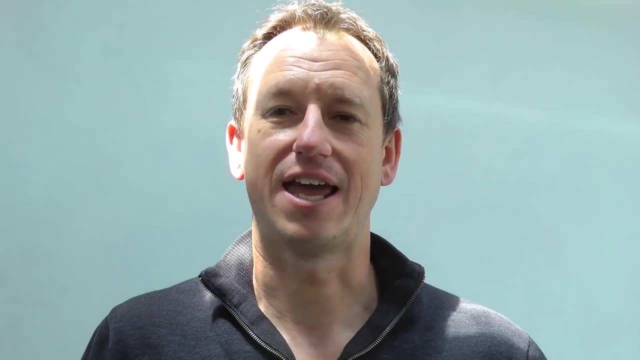 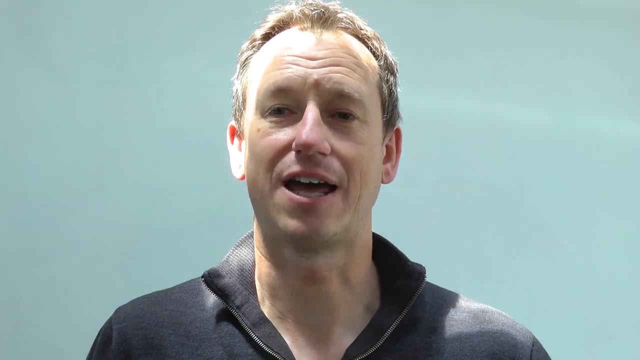 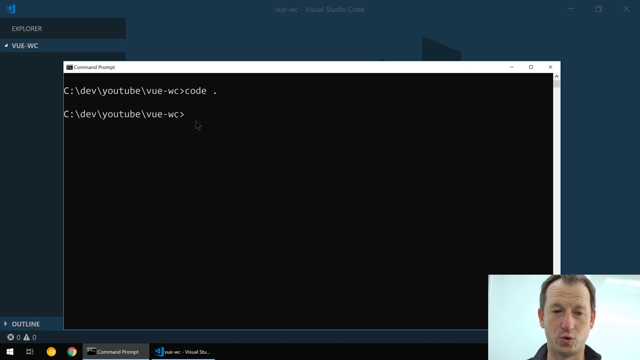 Today I'm gonna try with Vue, and we'll see how easy or how hard it is to put one together. So got Visual Studio Code open here. let's jump in and have a look. Okay, so the first thing I'm going to do here is get Vue installed, So let's. 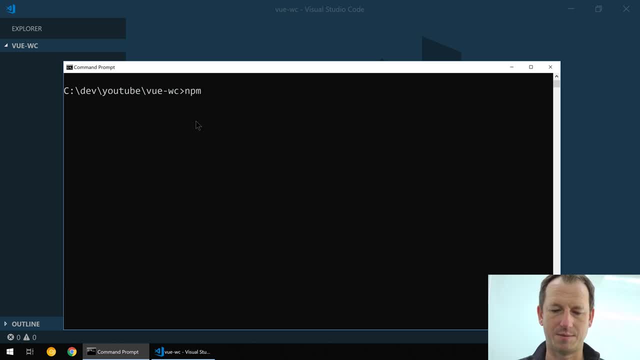 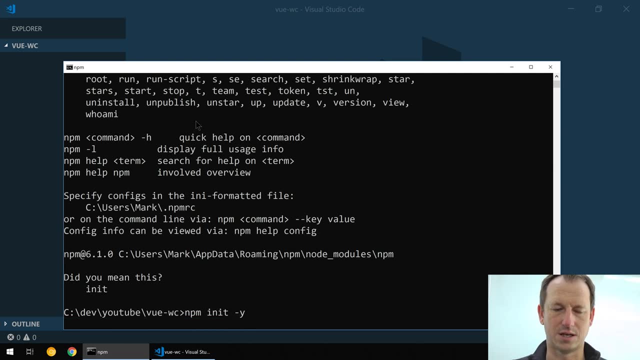 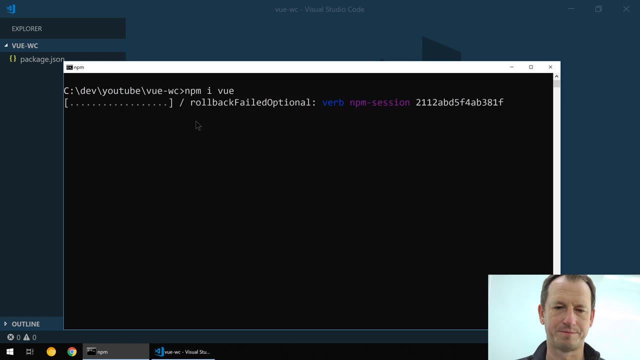 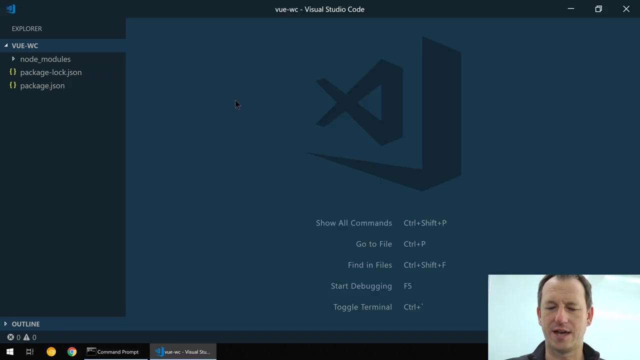 do an npm init like so, and then let's do an npm install of Vue, which should come in pretty quick Right now. with that installed, we'll come into VS Code and we're going to make a single file component that's literally just going to put up some text and a 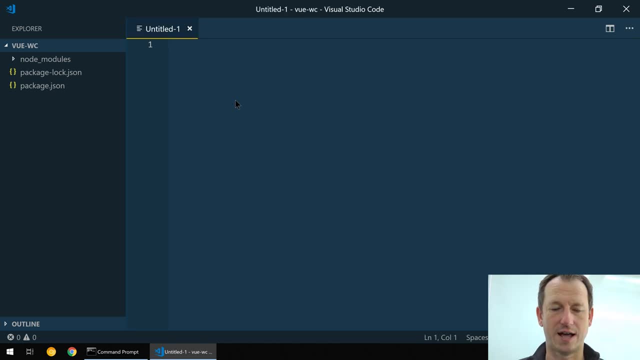 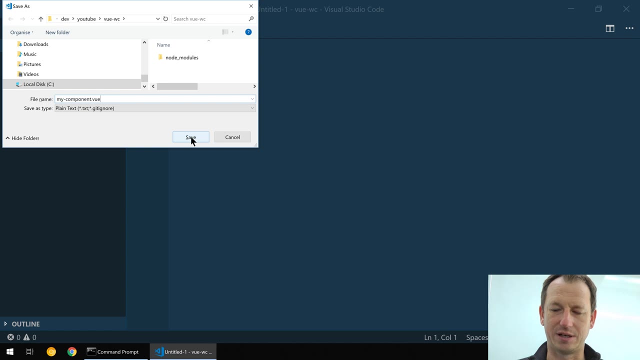 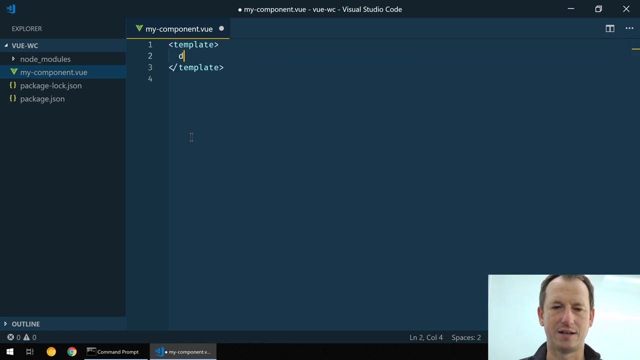 property for us. So let's create a new file in here and we'll call it my component. We'll put a hyphen in the name because web components need to have that hyphen there. So if we create a template here, then and a div. 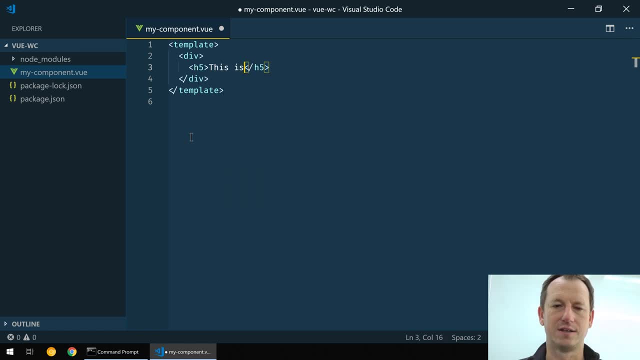 and then let's just put a header in and say: this is a web component created in Vue, Alright. and then underneath we'll say: have just another div. and we can say: let's just say my name is, and we'll have the name in here, just so that we can show. 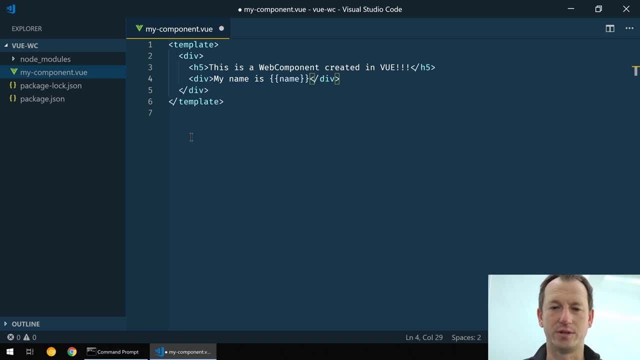 the use of attributes within a component. Alright, so that should be it for there. and if we just have a script now and we declare a props in Vue and we can declare our name property here and we can say it's a type string and we'll. 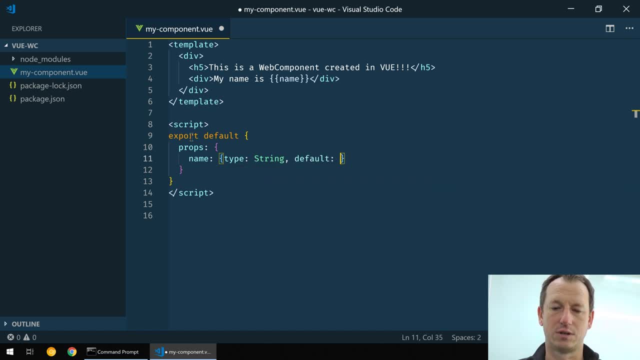 give it a default value and we'll just say mark in there. Okay, so that should be good for our component. Now we'll test this as a standalone Vue component just to start with, so I should just be able to do Vue serve here and get this coming up. 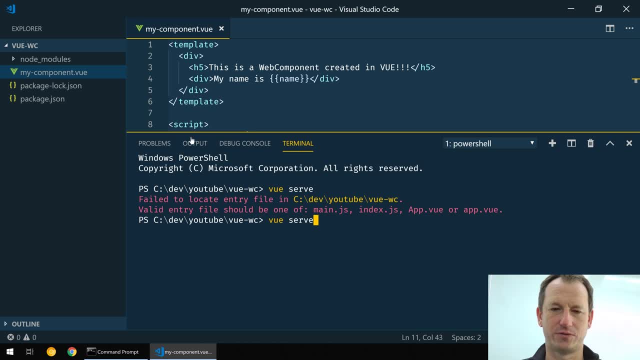 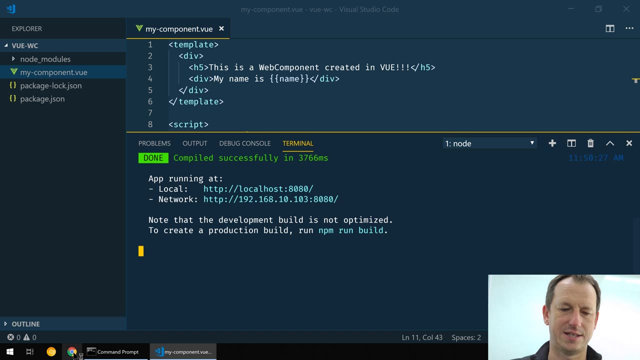 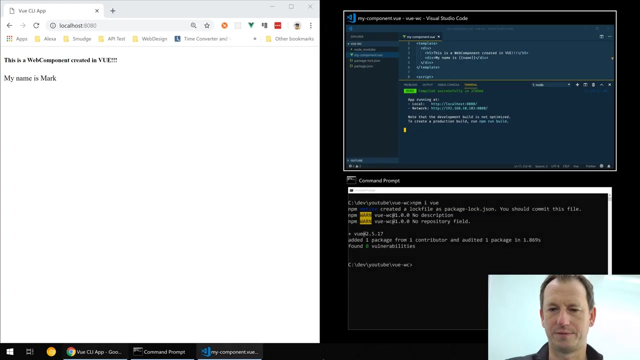 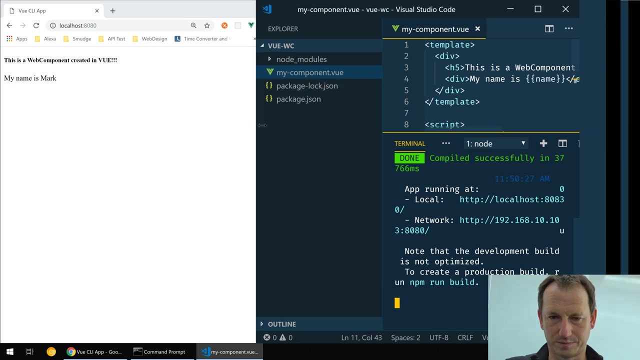 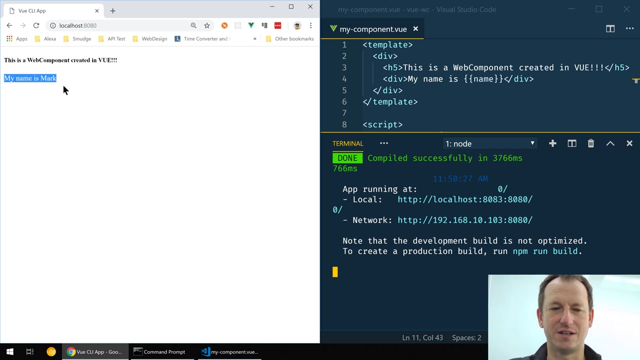 I think Vue serve my component dot Vue. okay, so on 8080.. Okay, and I'll just push this over here and make it a little bit smaller. Alright, so we can see our text coming up and then it's also displaying our property with its default value. Okay, now to use this as a web component. we. 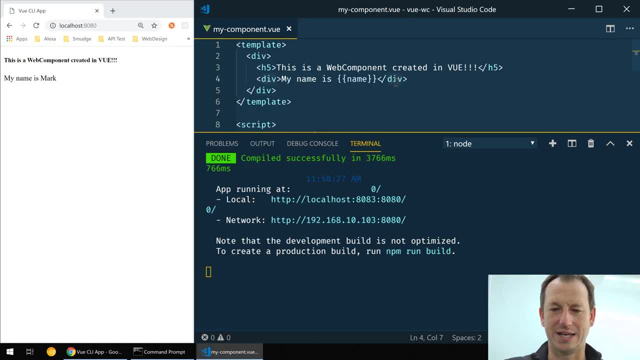 need to build it using the Vue CLI. So if you haven't got the Vue CLI installed, you need to do an npm, install global and then just Vue CLI. I've already got it on there, but that gives us the, the command I just used for Vue serve. It also gives. 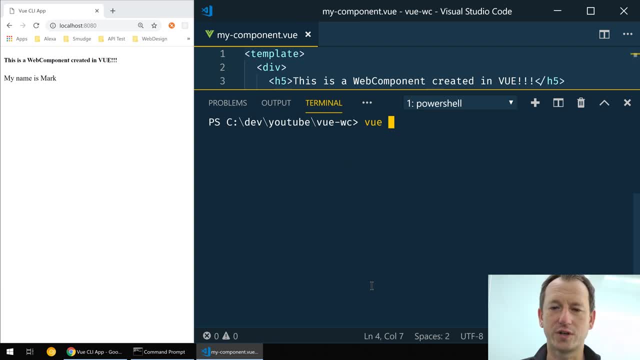 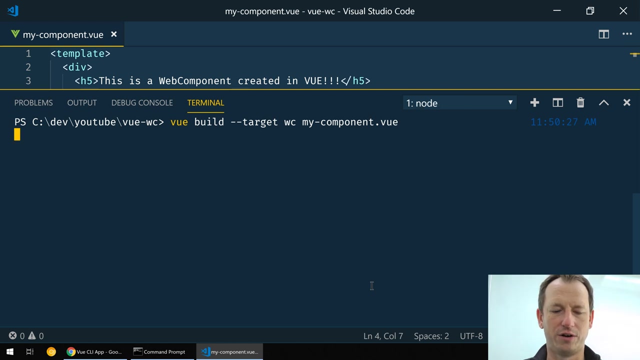 us Vue- this one is a little bit bigger- also gives us Vue build and we can say: we're going to target a web component and we want my component to be what we're building and just maximize it so we can see it. Okay, so if I kick that off, it's. 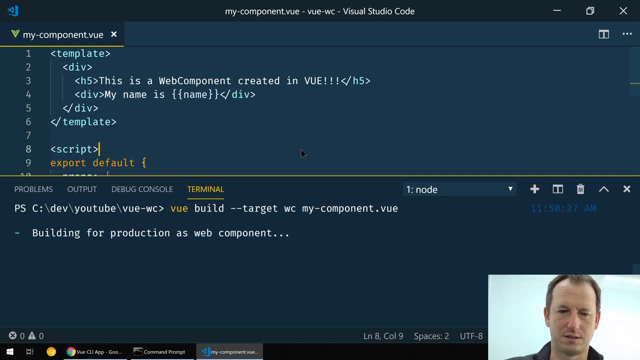 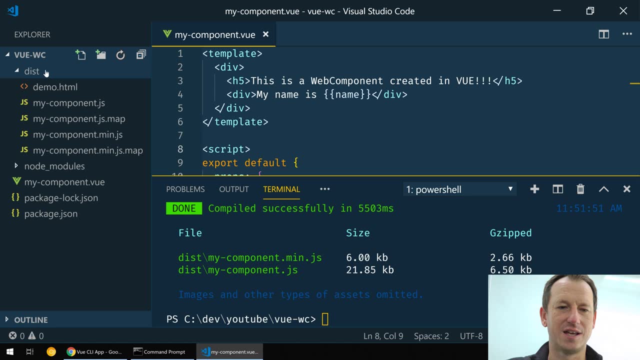 going to say: it's building that and I'll just bring this up here and you'll notice it created a dist folder here for us and in there we're going to be able to see that we've got our component wrapped with a Vue wrapper that turns it into a web. 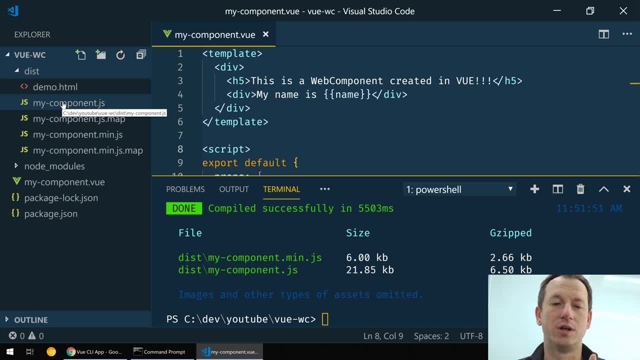 component. So it will. it will do a few things for us. It will place our content into the Shadow DOM, It will create the correct events for us and provide synchronization between our attributes and properties, And it will give us a style scoping. I'll try and show that in this demo as well. Okay, so let's. 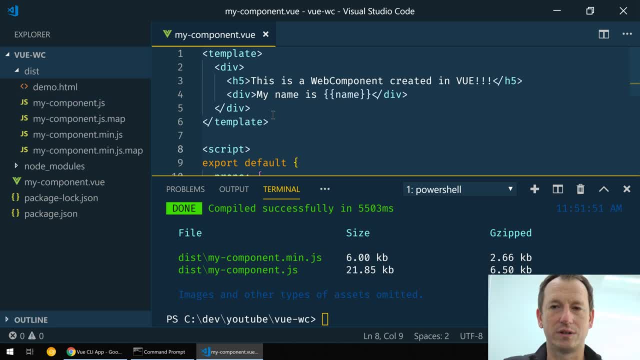 let's just um, let's try and use that now in another application. So normally you would probably publish this to npm. Once you've created a component, you publish it to npm and people will consume it from there. I'm not going to put it out to npm today, but I'm just going to do an npm link Actually, first. 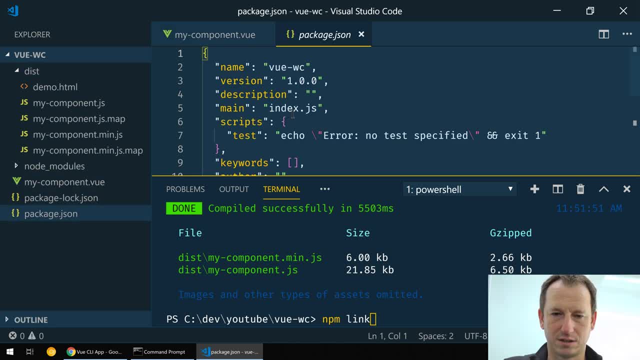 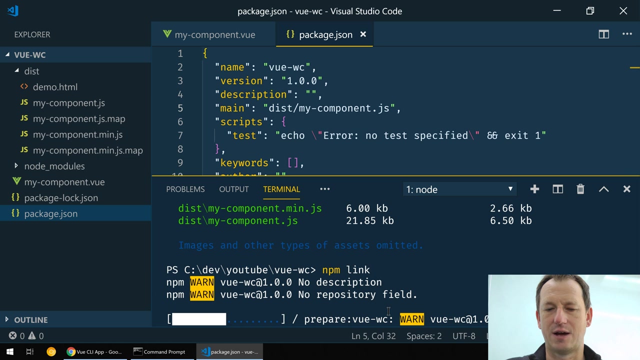 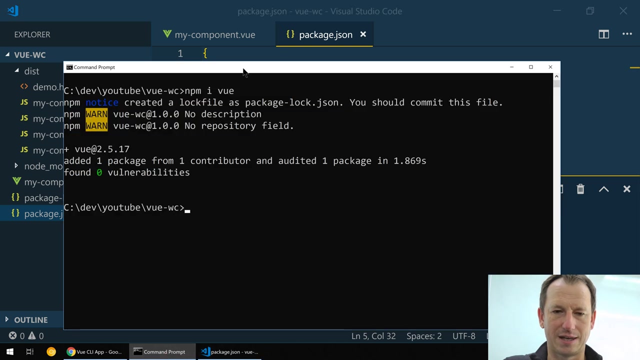 I'm just going to change the packagejson just so that we point to our component. So it's dist my componentjs and it will do an npm link, and that should allow us now to just pull this in without pushing it up to npm itself. All right, so let's come back into here. 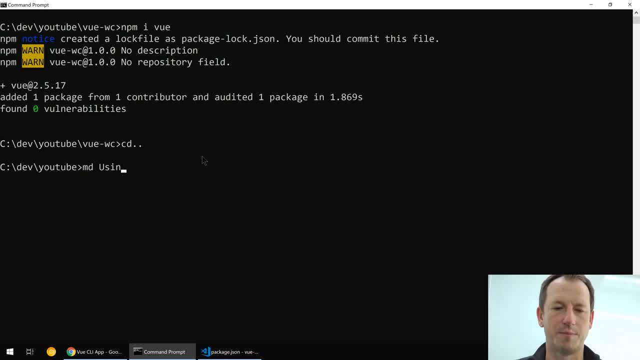 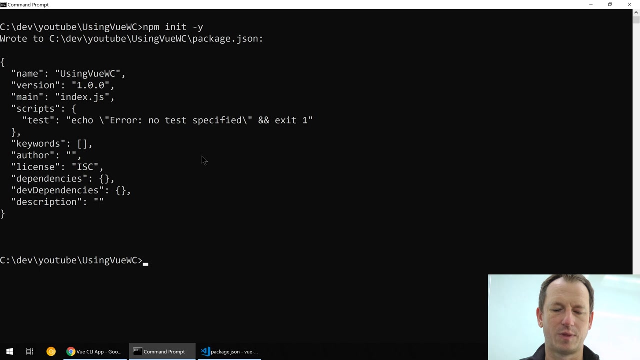 and we'll go and create a new directory, now called using view work component, which I've already done before. So let's try using VWC. Okay, all right, so in here, let's do an npm in it as well. well, and then we we're still going to need to have view, but i'm not going to install it as such. 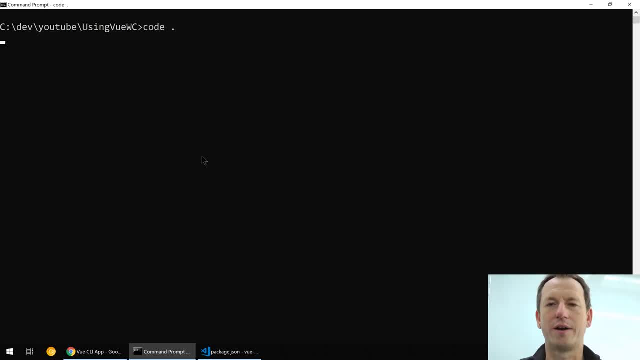 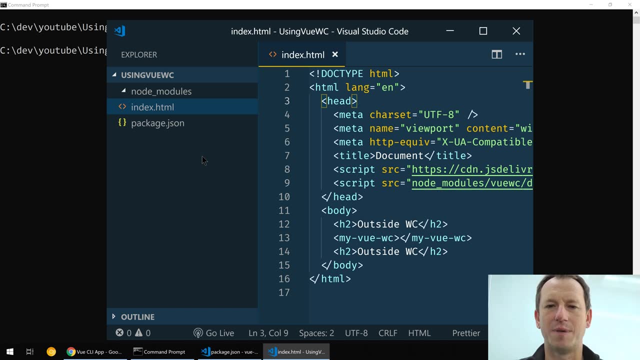 i'm just going to pull it from the cdn. so our our component still uses view internally. so we will still need to include view and it doesn't embed it in the bundle because you might be using multiple versions. you might have multiple view web components. you still want that duplicated in. 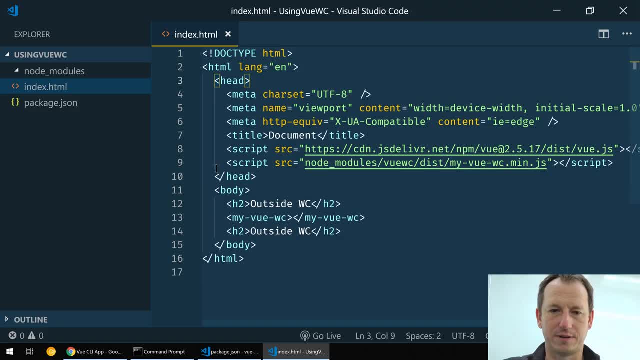 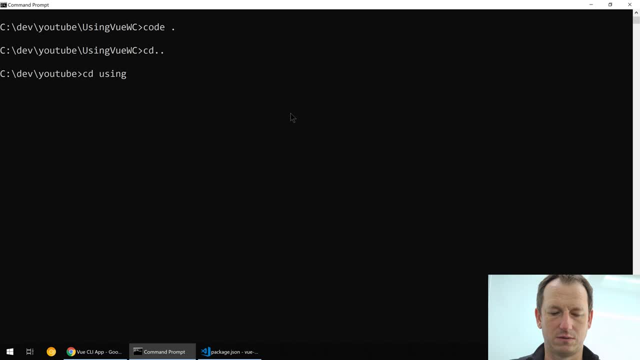 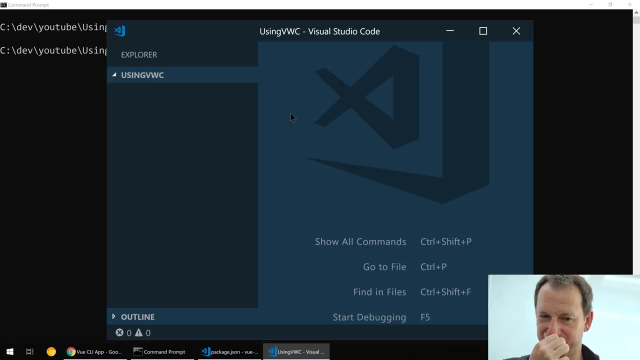 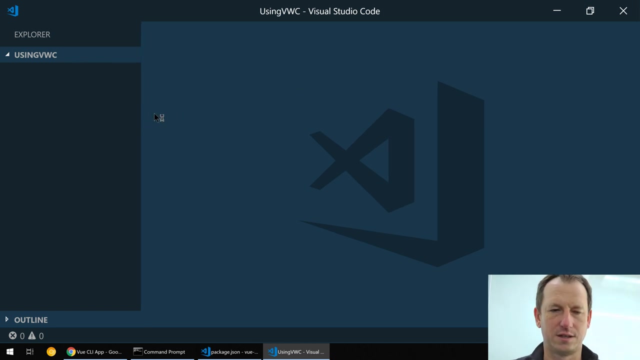 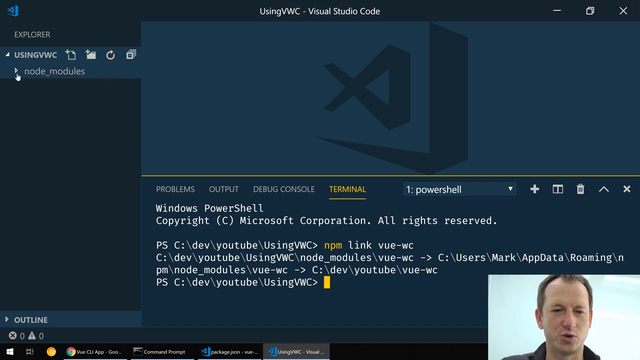 there, um, so if i've come to the wrong one, let's go using vwc and open up code there. okay, so now we've got a blank one, um, right, right, let's. uh, let's pull that in. so if we do npm on link and view wc, that should give us access to the component. you see, it created the node modules. 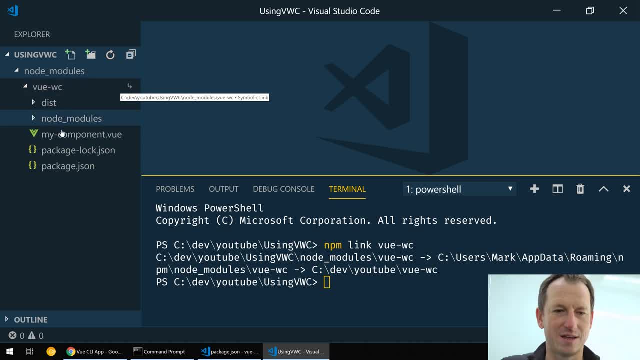 here and it's a shortcut denoted by that there. back to our component. so we're going to try and pull in, uh, this file here, our my componentsjs. okay, so i'm going to create it there. i create an indexhtml here and just put some boilerplate code on. 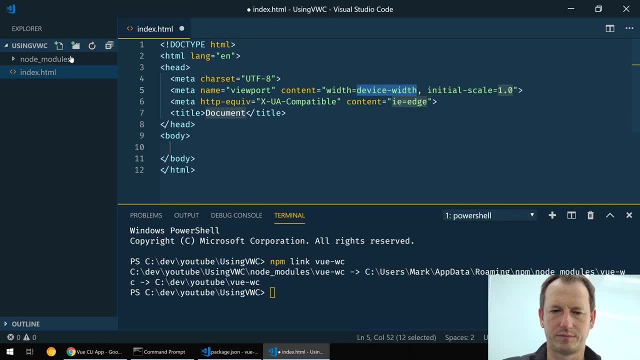 okay, so we'll have a script and the first thing we'll do is pull in the view itself and we'll get that from unpackagecom and view, so you can install this with npm or we can just use the cdn here for this um, this, this example, and then we'll pull in. 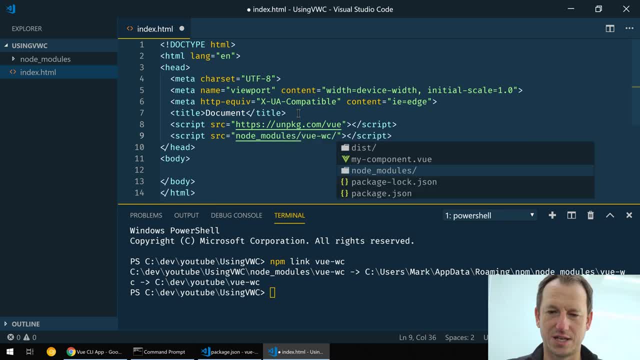 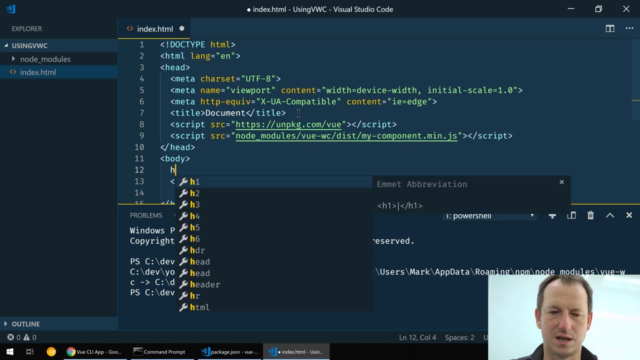 our component, which is in node modules, view wc. it's in the dist folder and we use the minified one, and then we should just be able to use my component down here, like so, and i'll just put a little header above it. view component be below: okay. 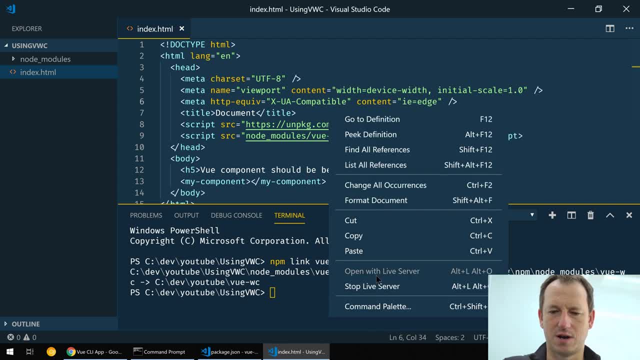 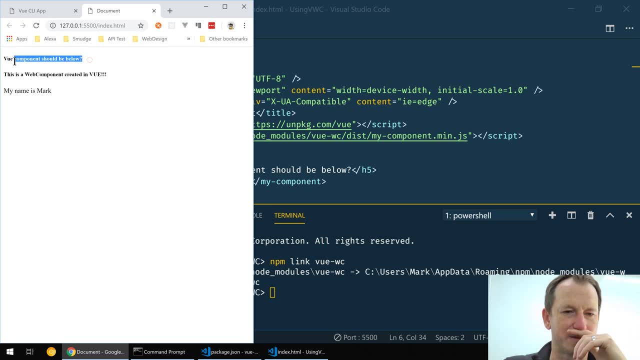 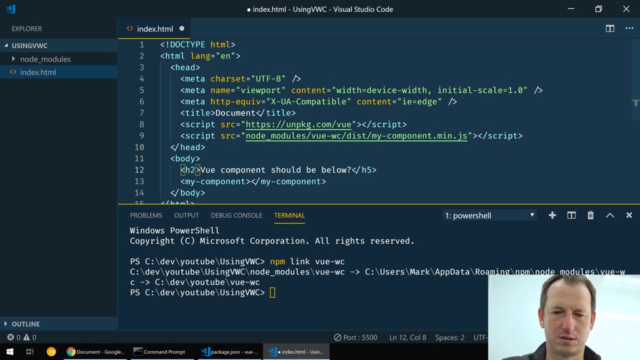 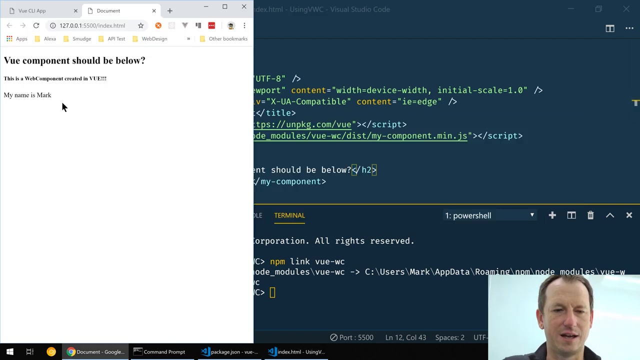 right, so let's give that a run if i do an open live server on that. okay, so there's our text from our that we typed in here in that h5, just going to make that a bit bigger, just so we can see things, okay, and then here is the web component that we saw earlier. 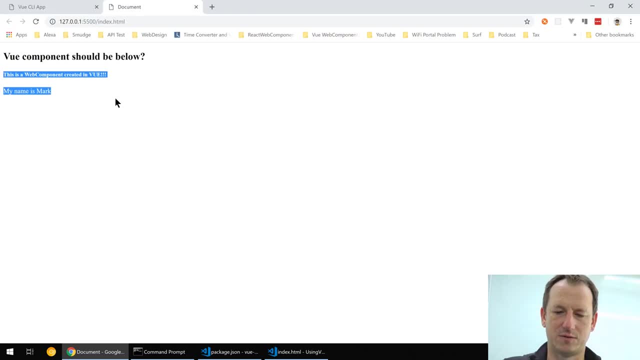 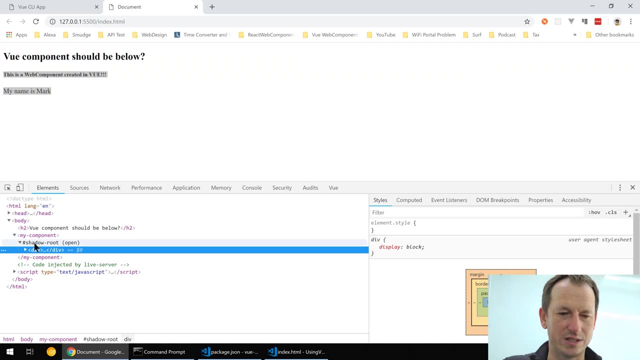 so let's maximize that and we'll just put a little header above it and open up dev tools a minute. so if we click on this now and we look into the elements, we can see my component has got a shadow root, so it's, it's turned into a web component for us. 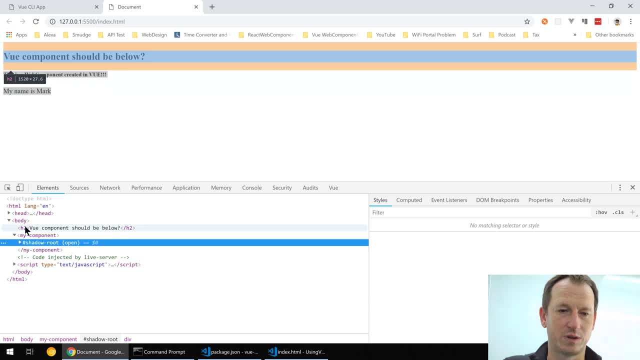 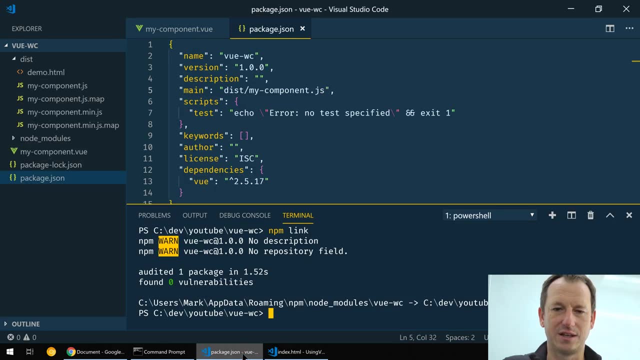 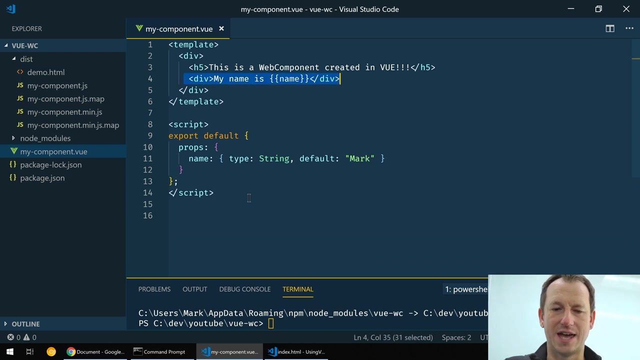 and then in there we'll see our actual component right. so what else can we do just to check that it's working as we'd expect a web component to, and one thing we can do there then is let's set some style on it. so it's using a div in here for the name section. you know, if i set up. 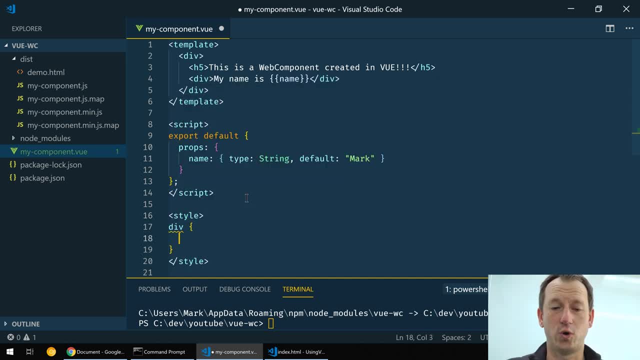 a style here and i said: right, i'm just, i'm going to set for all divs. so i'm going to set a border, pixel black, and hopefully this is going to show the encapsulation for us, because if you did that style anywhere else, uh, in an app, in a web app, it's going to affect everything. 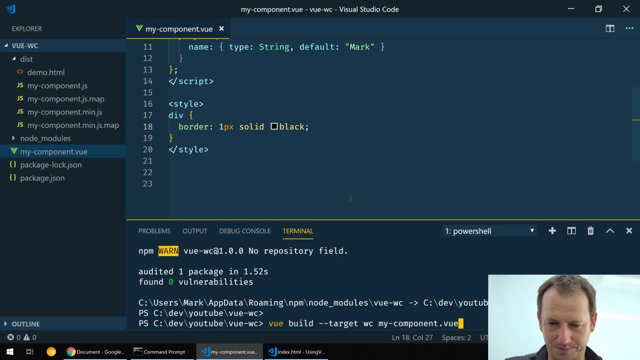 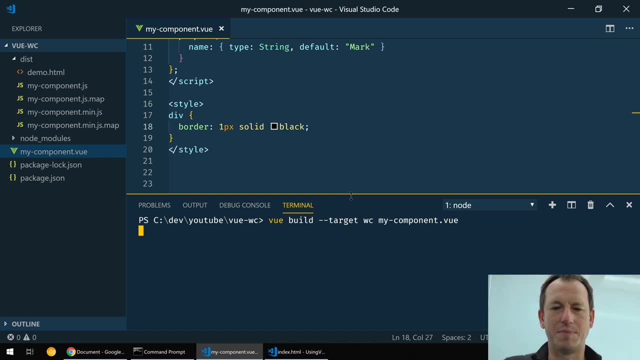 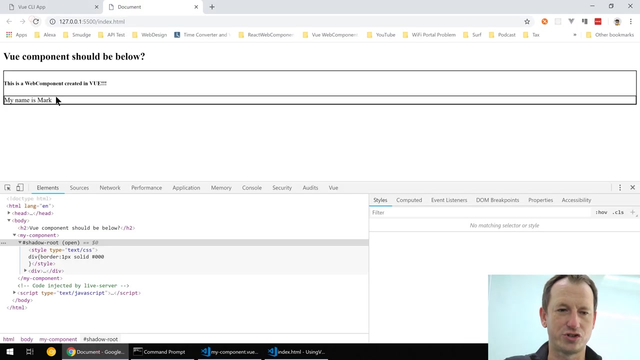 so if i rebuild that, just bring this up just so we can see. okay, so we give that a rebuild with this new style incorporated. and then if i come back to my page here and just refresh, we can see we've got a border around the divs of our component. 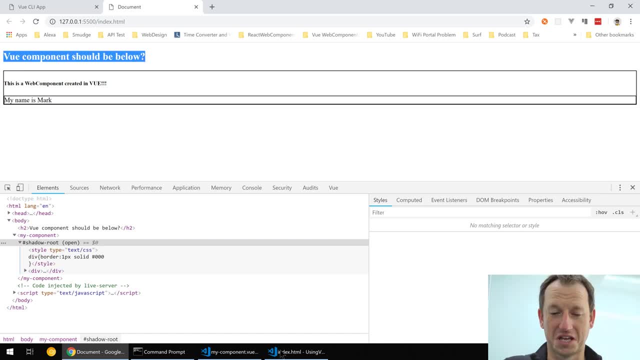 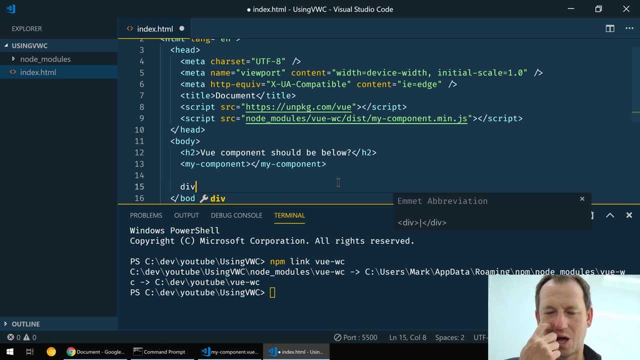 but we haven't got anything around this one, and we shouldn't because that's a header, so let me put a div in here. so we're back in our web page that is using our component now, and if i say this should not, should not- have a border. 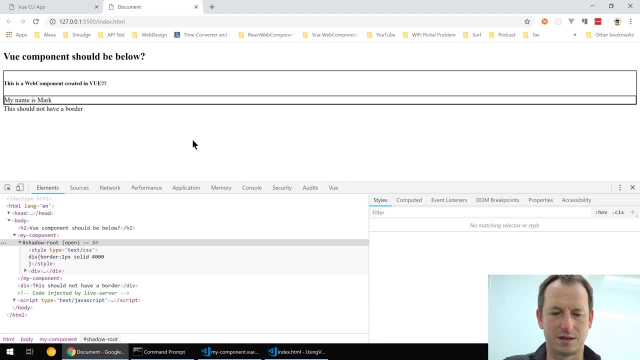 and if i save that off, we flick back, we can see there's no border around this. so the the div style is only affecting our web component, and this is one of the great things about web components is that style encapsulation, so the view wrapper is is doing its job. uh, correctly there, um, and then. so just one more thing, just to. 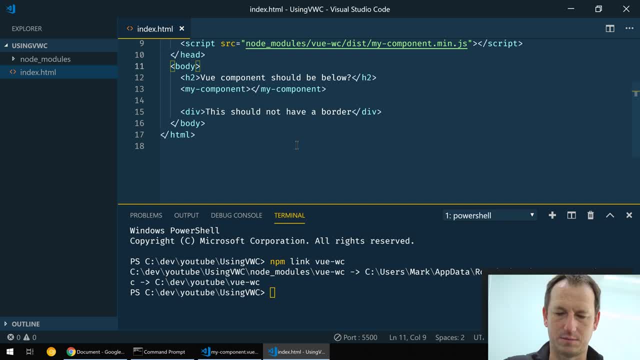 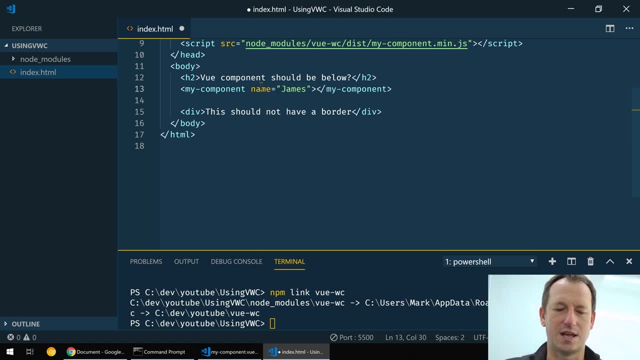 i'm sure that it's working correctly. i'll go into our component and let's, let's specify: the name is actually now james and hopefully that should then get um synced to our property on the component and that should now come up in here. so it's like this because it's got a live refresh, it's already. 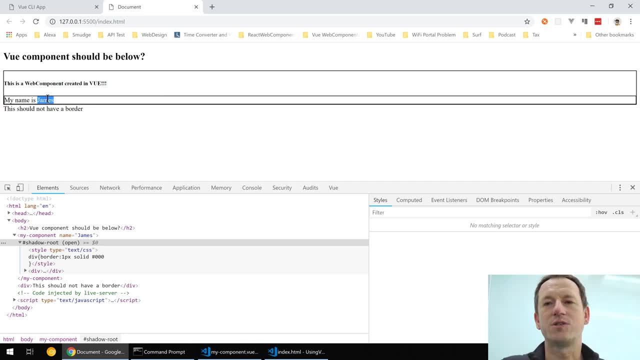 got my name is james on there, um, so there's other things we can do to show that it's uh operating as a weapon component, but i think that's- you know, that's pretty good and that was incredibly uh easy as well. if i come back in here now, um, and let's have a a little check as well, 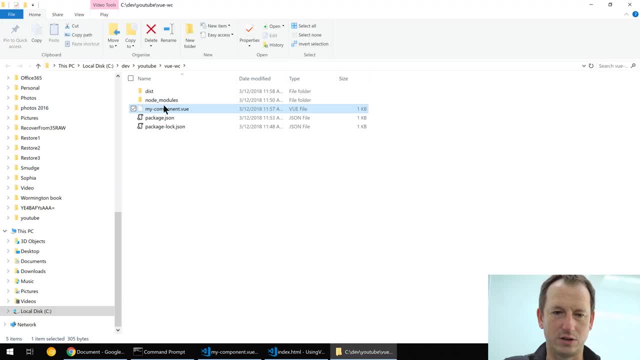 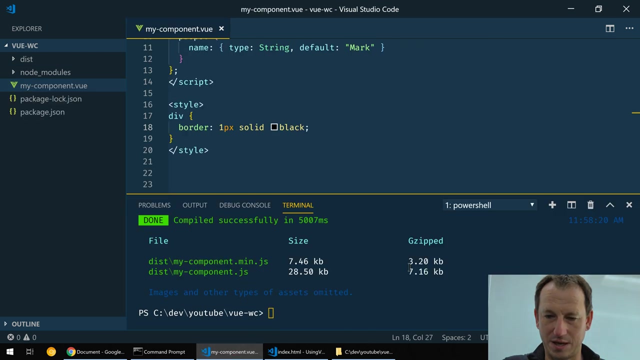 in explorer. if we look at dist and look at these sizes, the minified one is 8k. so you know pretty good, you know it'll probably only get smaller um. and if we look actually what it would be g zipped like um into here, we look at what it would be. you know, once it's g zipped this component would be. 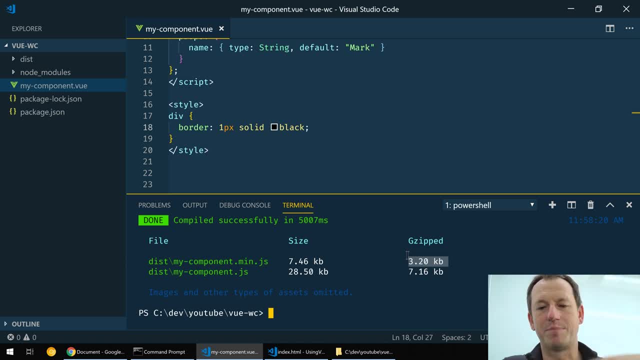 down to 3.2. we've still got view on top of that, but we'd only have one view for for all of those components. um, so there you go. that's how to create a web component in view. as i say, i'm going to do a. 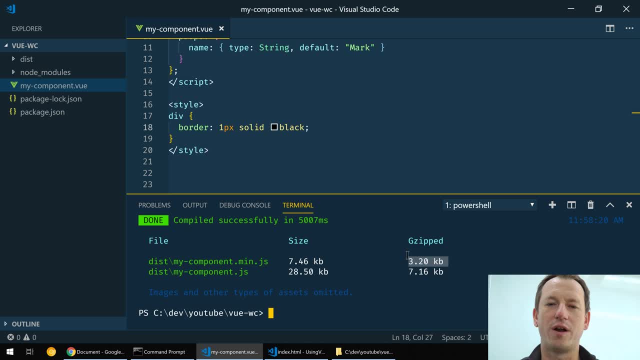 few of these. i'm going to try and do a react one and an angular one, and then maybe some others as well. see how easy, hard it is in those as well. um, thanks very much for watching. if you want to see those and, uh, want an alert, then click on that subscribe button and give us a thumbs up, thumbs. 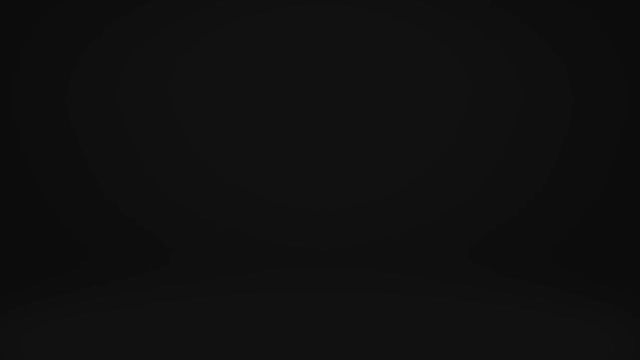 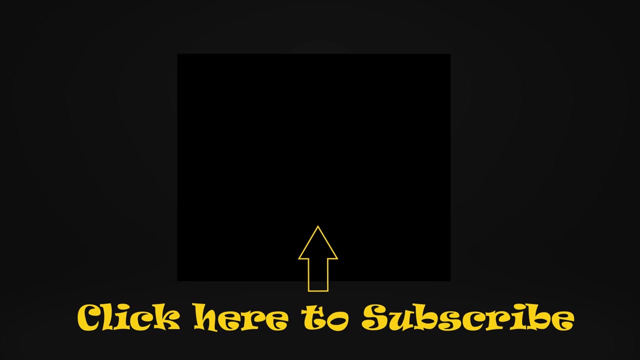 down and i'll see you next time. thanks, bye you.